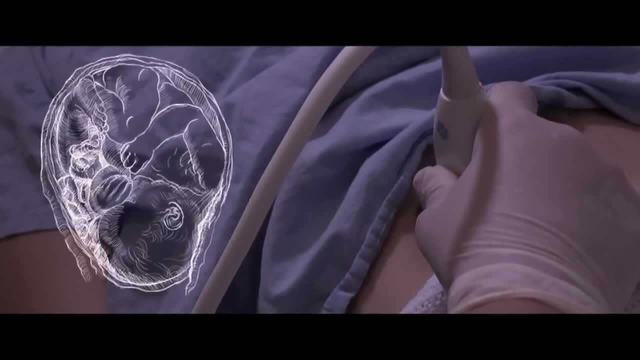 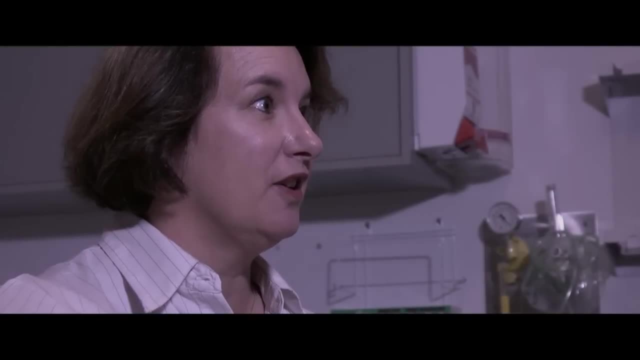 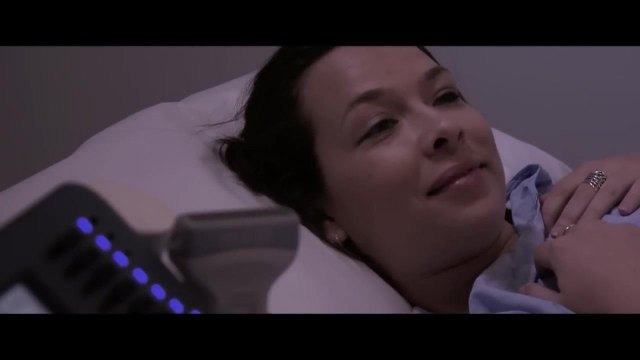 imaging experience is one in which we have no memory. an ultrasound examination during our mother's pregnancy. It is used to assess how old we are, how fast we are growing and if we are likely to be a healthy baby. Based on this examination, doctors make critical decisions. 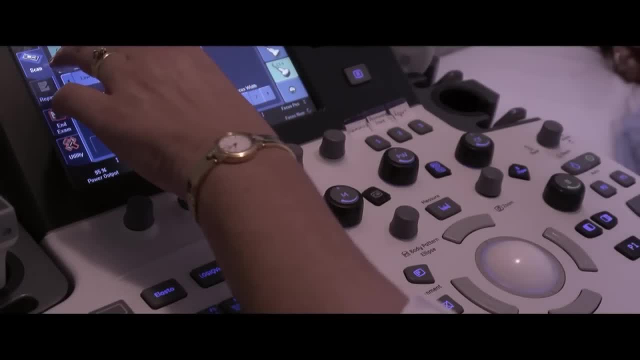 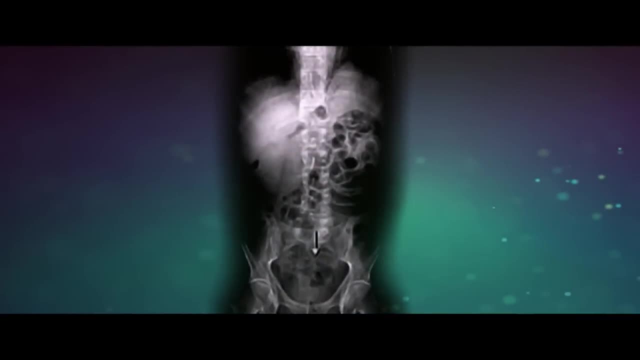 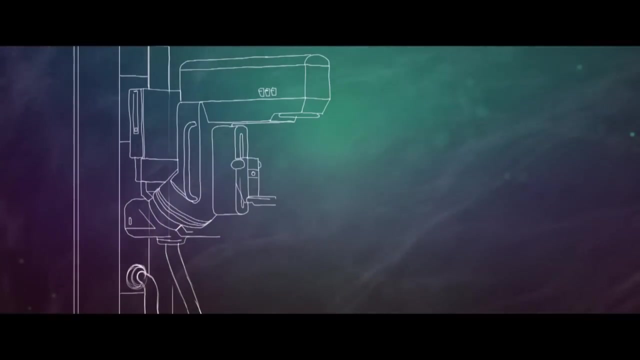 about our health and the health of our mother. Then, during our life journey, we have x-rays of our teeth or a CT x-ray for abdominal pain. It may be bone scans for stress fractures or routine mammograms as a screening tool. My name is Professor Graeme Galloway and I am Group Leader. 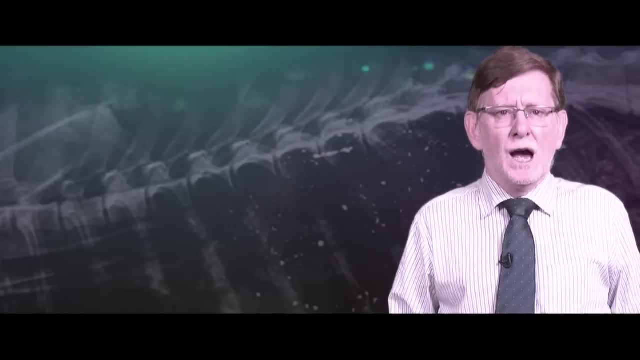 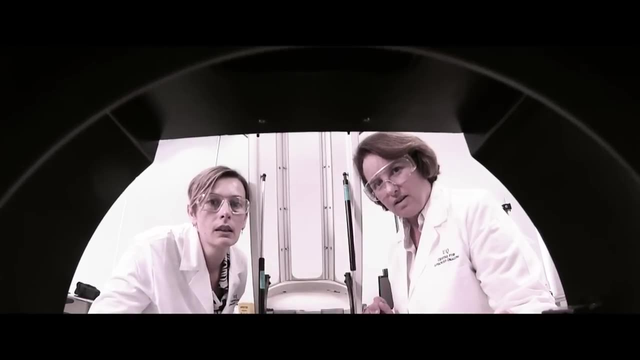 for Biomedical Imaging at the Centre for Advanced Imaging at the University of Queensland. In this course, we will introduce you to the fundamental principles of all these imaging technologies and also give you a tantalising overview of the medical world. In this course, we will introduce 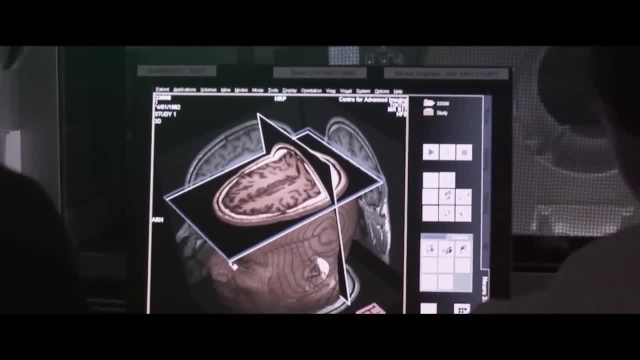 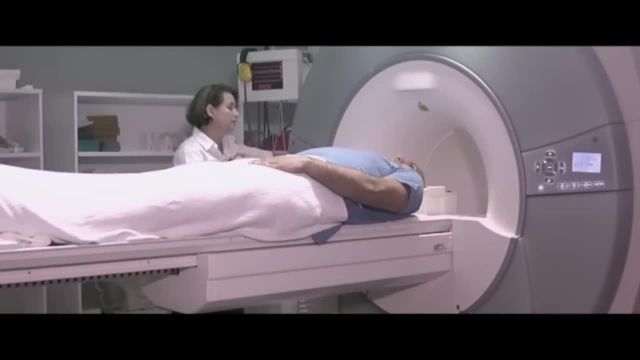 you to the fundamental principles of all these imaging technologies and also give you a tantalising glimpse of the future of imaging. We will see how these different technologies complement each other and why we need so many different tools. We will find out more about magnetic resonance imaging. 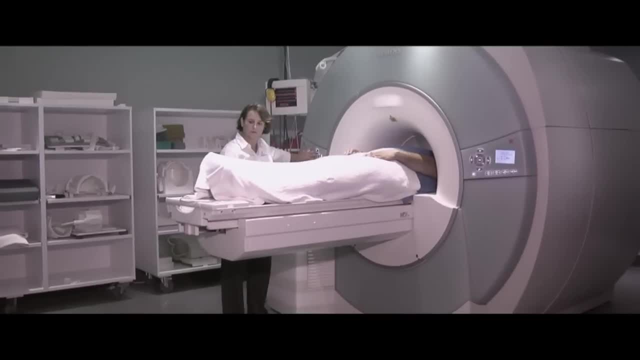 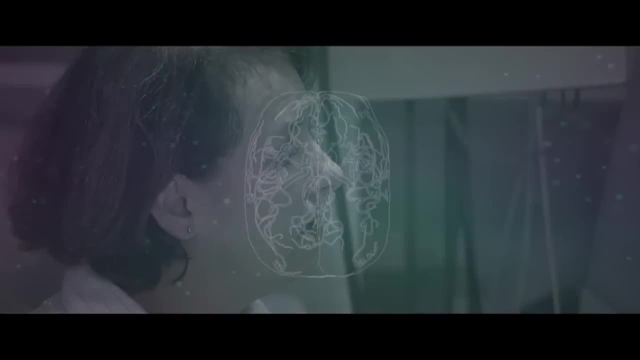 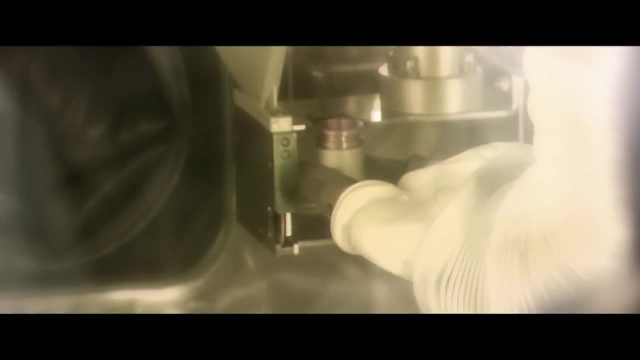 and how we increase the contrast of the image to help in the diagnosis. You might have heard about functional MRI and its role in neuroscience and psychology. Can we really see what you are thinking? We will do some chemistry- chemistry using sophisticated automated equipment. 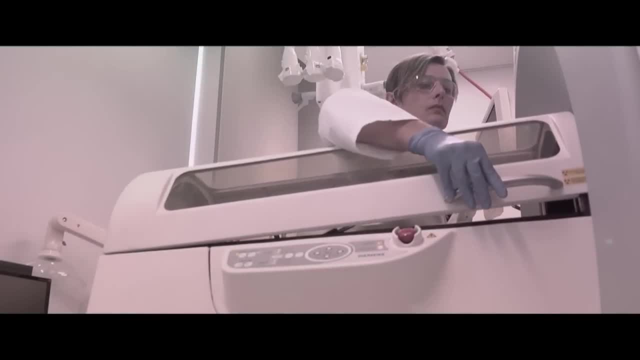 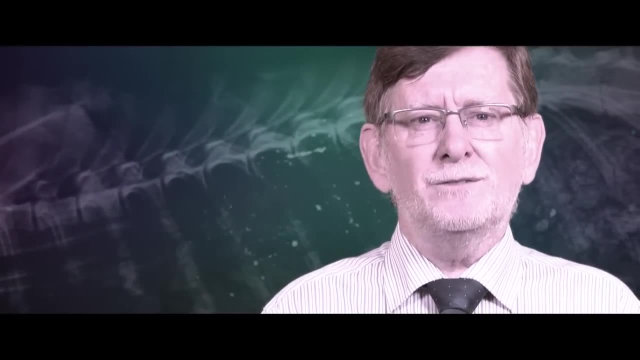 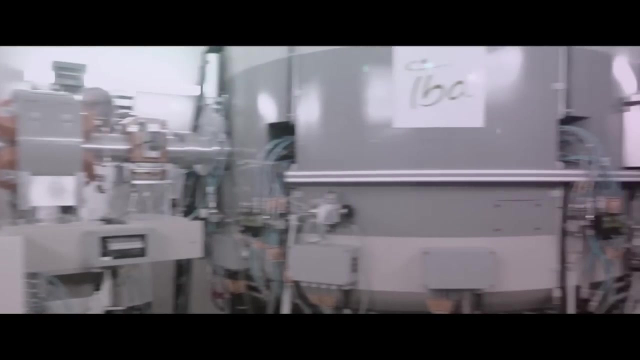 and you will learn about radioisotopes, cyclotrons and hot cells. As you'd have guessed, all these techniques generate a huge amount of data, so much so that we're talking about an explosion of information. The challenge is to store and analyze this information. 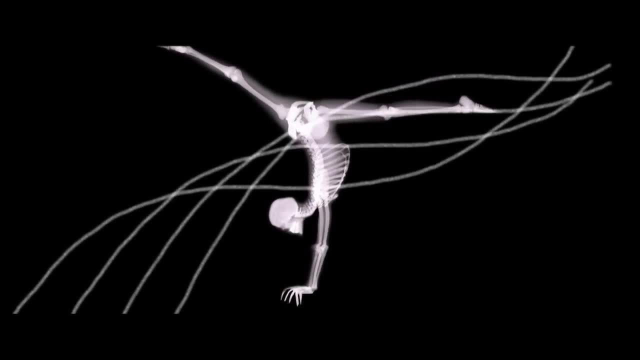 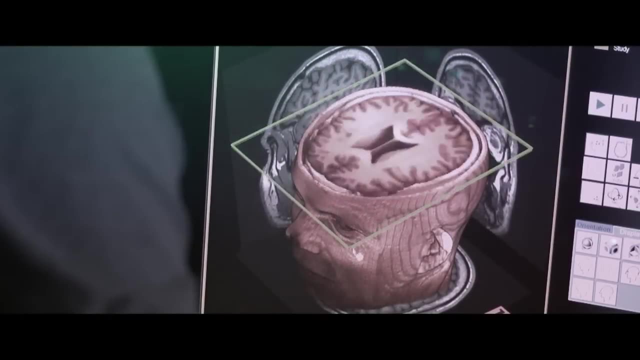 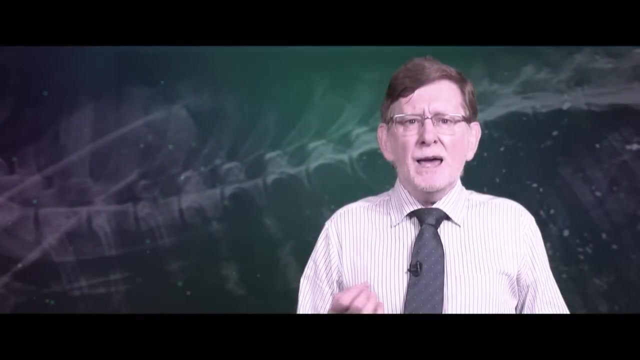 This is where visualization becomes so important. from simple two-dimensional black and white images to spectacular 3D dynamic color images you can fly through. So who will be interested in this course? It may be that you are concerned about your health or the health of one of your loved ones.